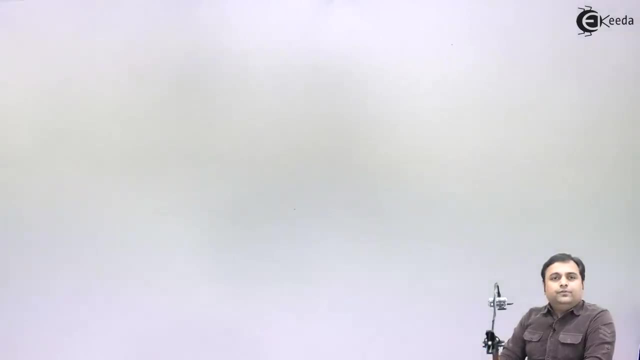 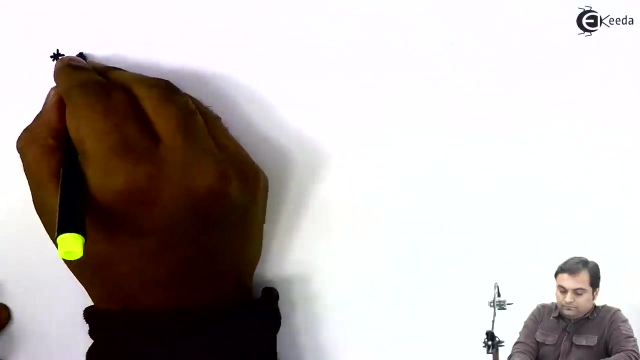 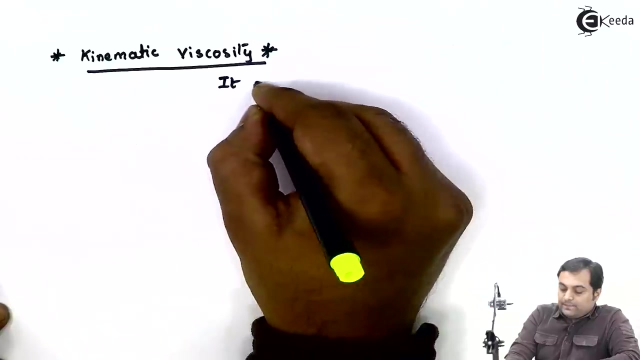 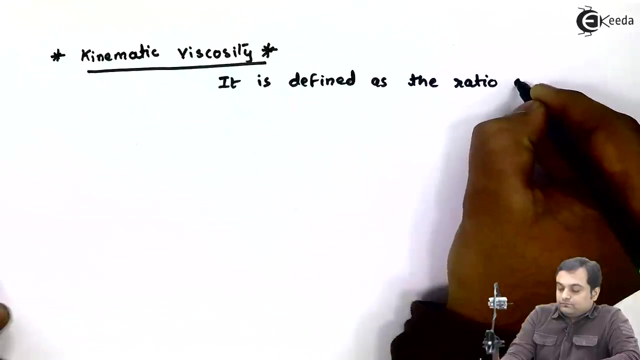 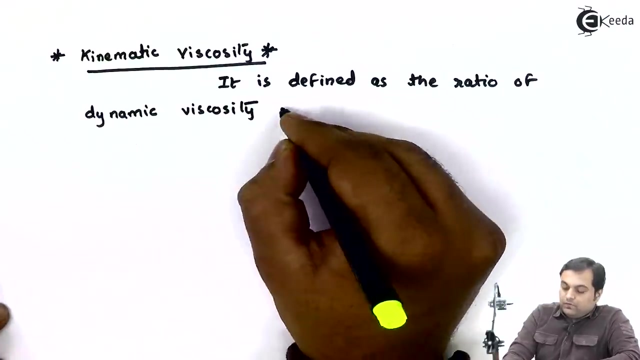 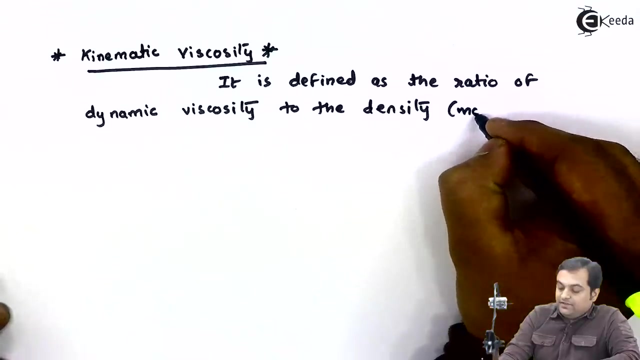 Hello friends, in this video we will see the definition of kinematic viscosity and its unit. So let us start with it. Kinematic viscosity: it is defined as the ratio of dynamic viscosity to the density. or here, if I write density, it is mass density. 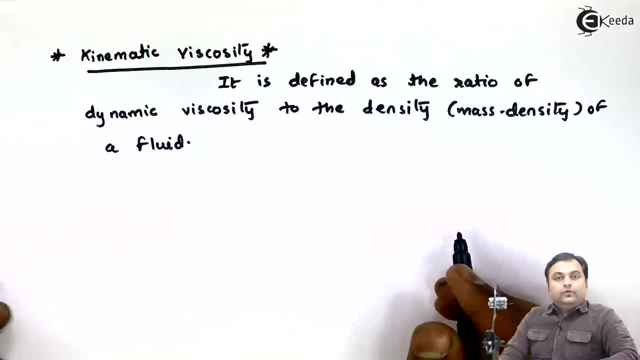 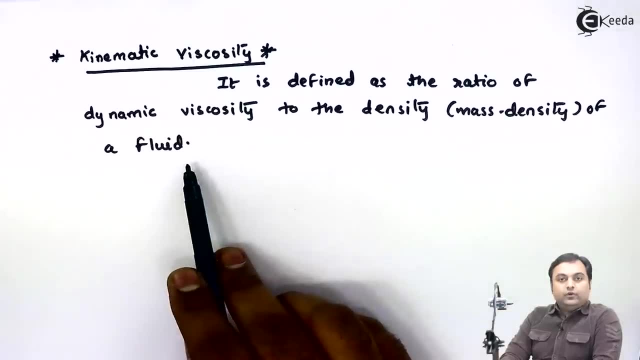 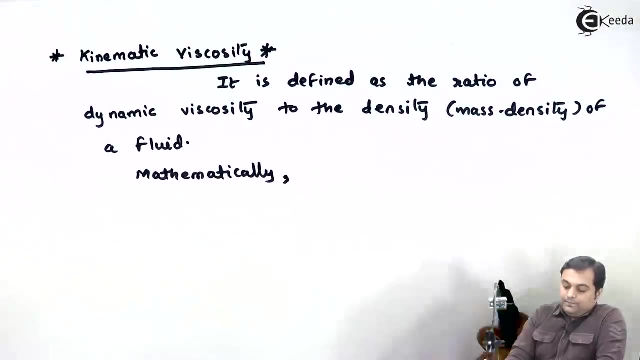 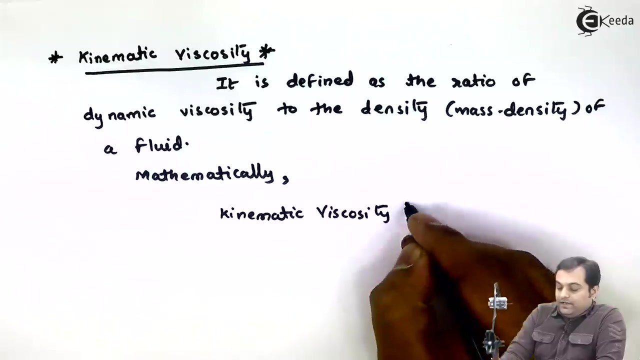 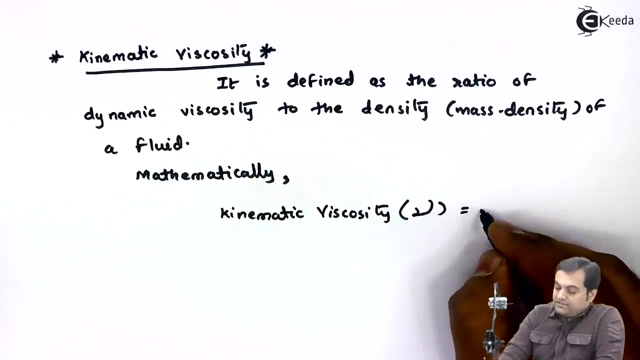 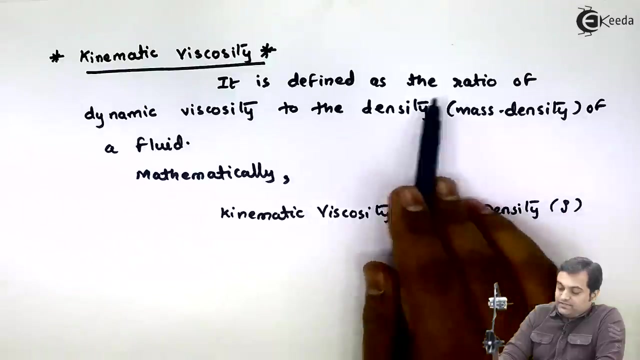 of a fluid, So kinematic viscosity. it is defined as a ratio of dynamic viscosity to the density of fluid. so mathematically kinematic viscosity it is denoted by Greek letter NEO, and this is given by mass density, or simply density, which is rho. it is dynamic viscosity to density. 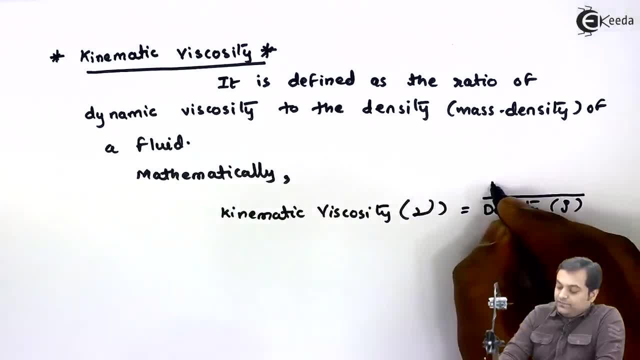 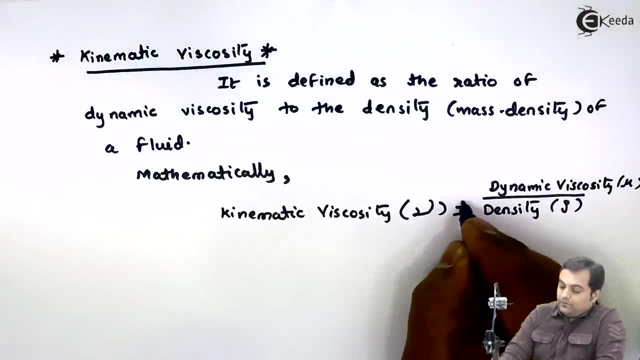 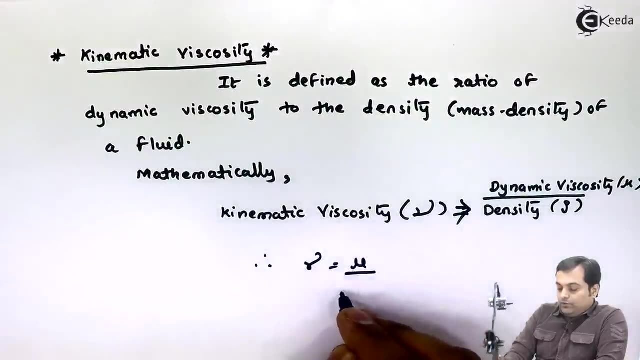 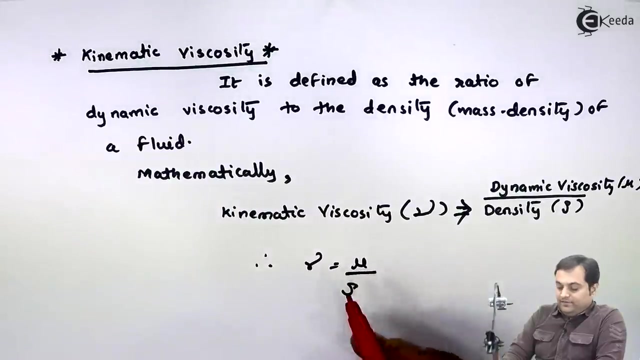 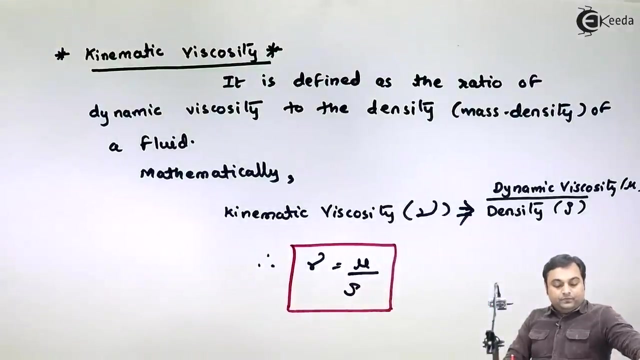 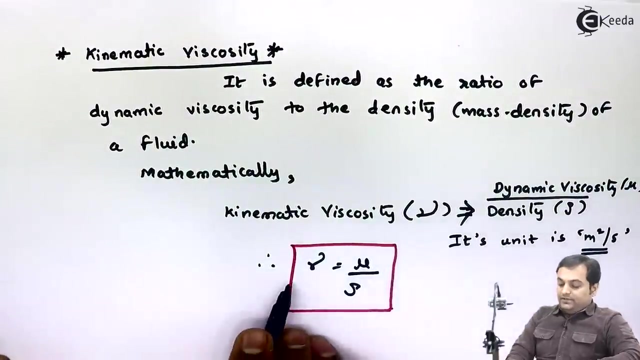 so here I have this as dynamic viscosity, that is, mu upon density. so therefore NEO, it will be equal to mu upon density. So here I am also seeing the relation between kinematic viscosity and dynamic viscosity. Next here its unit is. it is m2 per second, and sometimes kinematic viscosity is given. 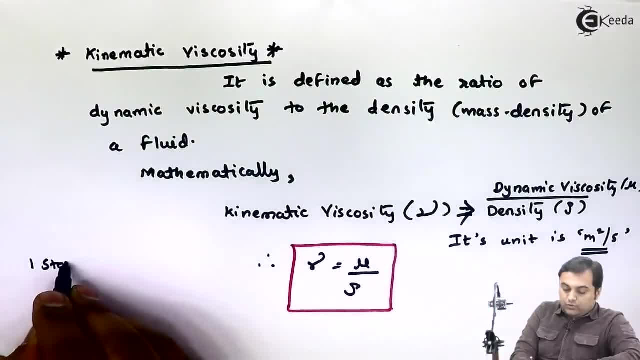 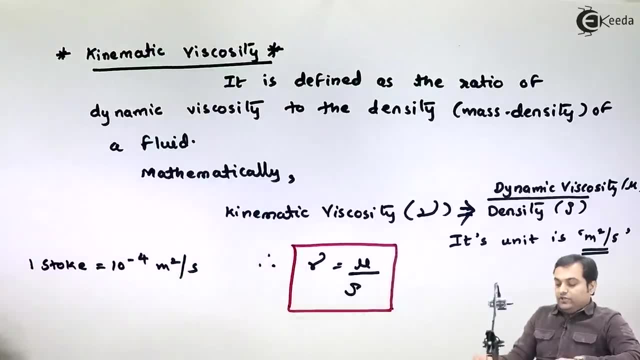 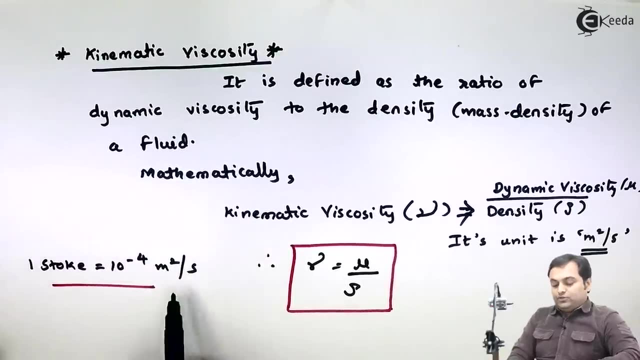 in the form of Stokes, stokes. so one stoke is equal to 10. raise to minus 4 meter square per second. so if in the question they have given kinematic viscosity in the form of stoke, that we can convert it into meter square. 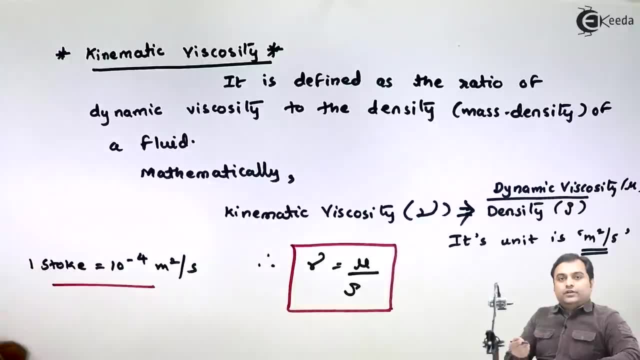 per second and use. it means we have to convert stoke into meter square per second by multiplying it by 10, raise to minus 4. so here in this video we have seen kinematic viscosity with its relation and its unit.